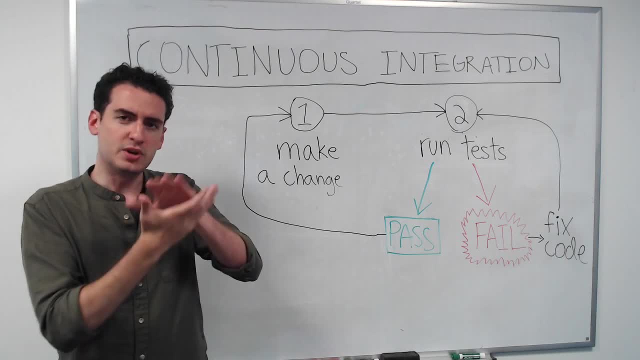 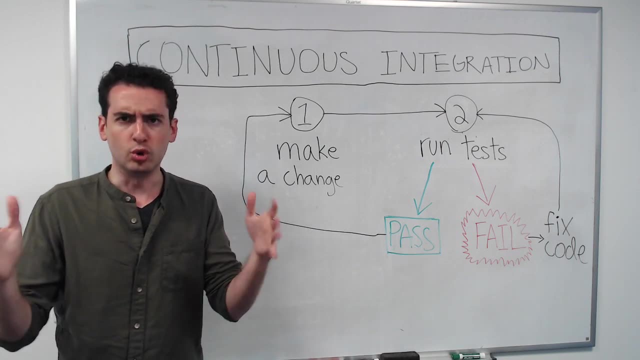 After each change that they're making, there's a suite of tests that runs automatically that checks the code for any bugs or errors or anything like that. Cool. so what does that look like in practice? I've drawn this beautiful flowchart up here for you. 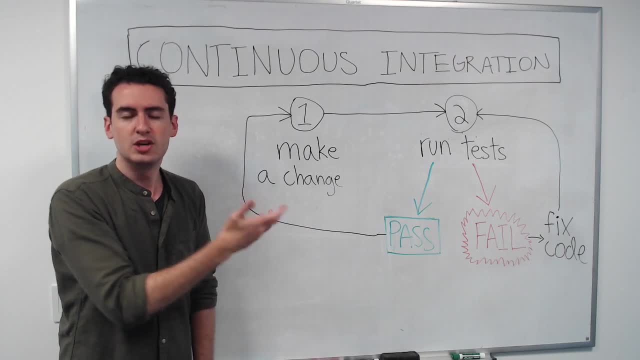 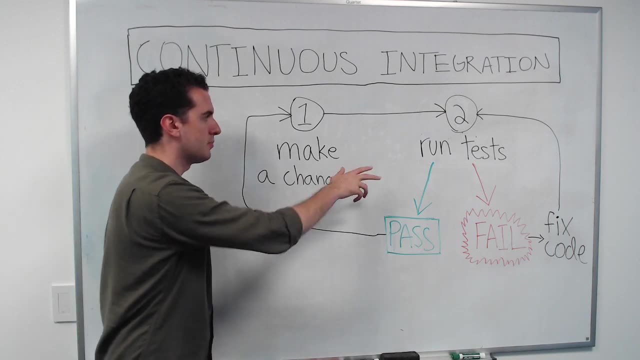 Step one is you make a change, and this is something maybe on GitHub. You make a future branch, you push it up, submit a pull request. That's the change that I'm talking about here. okay, Push that up, then you run your tests automatically and that's pretty important.